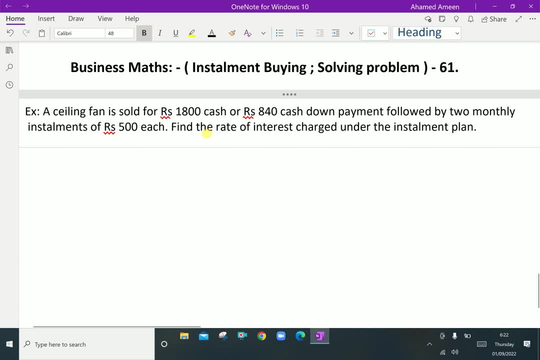 Find the rate of interest charged under this installment plan. Look at this here. If you buy a fan by cash price, it is Rs 1,800, or by installment, we have to pay first cash down payment for Rs 840 and remaining two installments for Rs 500 each. 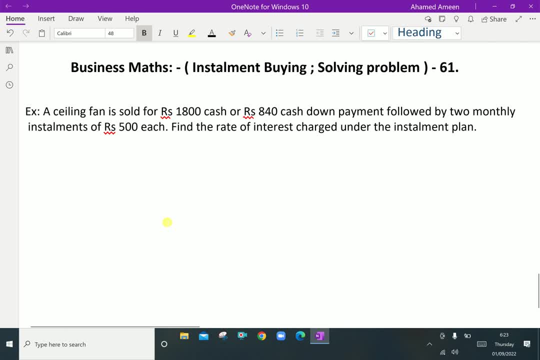 Each month you have to pay. Thank you. Now cash price of ceiling fan is equal to Rs 1,800.. Then cash down payment. Cash down payment is Rs 840.. Then remaining balance is Rs 960.. 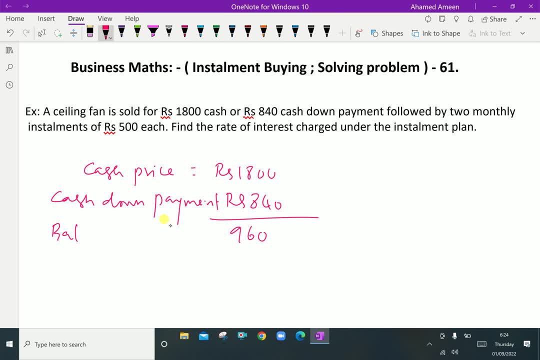 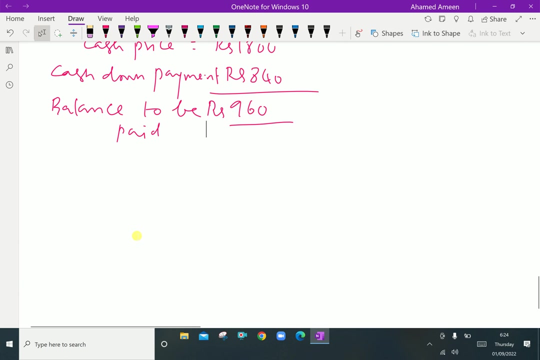 That is balance to be paid. That is balance to be paid. That is Rs 960.. Here, let the rate of interest charged by this plan. Rate of interest charged is equal to R% per annum. Then here Rase at. rate of interest charge is equal to R% per annum. 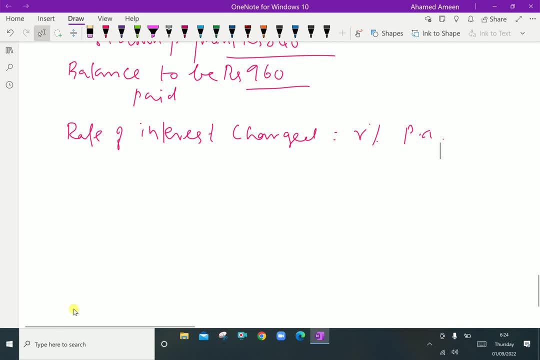 That is RSE per annum. Rate of interest keys. Rate of interest keys. amount of interest keys. kannibalsharingcom- 받 Lang concurrency Bond online. Googleастиcom. At the end of two months it will become Rs 6 うm. 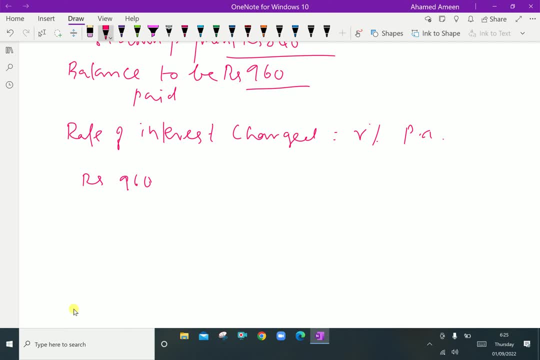 ande The amount of interest that is earned at the end of two months will become Rs 6 U Um. Can someone sign the card? aye, I don't know, sir. Here they are. So your card is Arab入 carriage format. 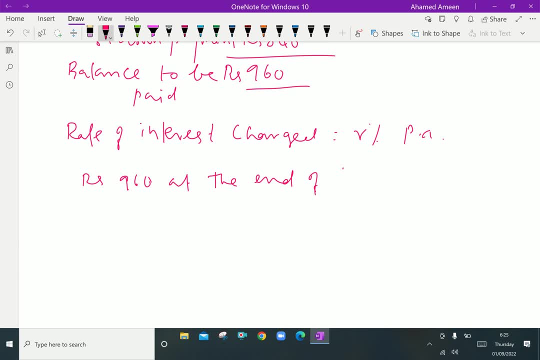 end of two months become two months. become here, that is 960 plus 960 of R percent R by 100 for two months, 2 by 12 for year Now, which is simplified, is 960, then it is equal 16 R by 10, that is the equation 1.. 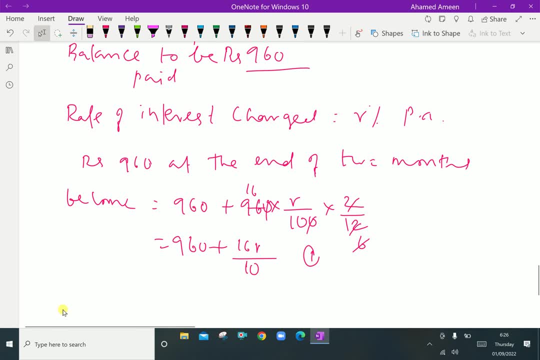 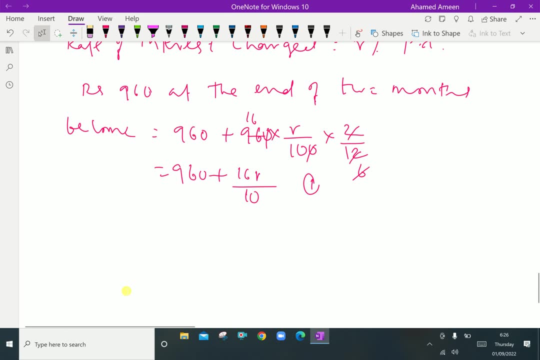 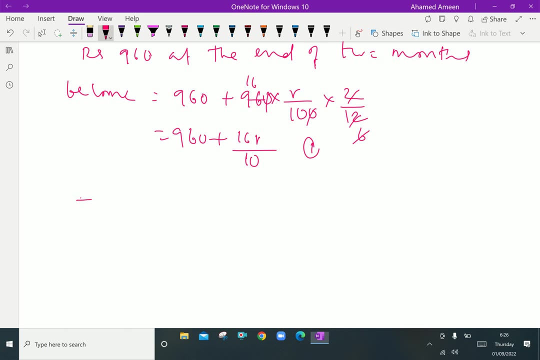 Now, here you have 500 to be paid, 500 at the end of rupees 500, 500 at the end of take off. 500 at the end of two months will become two months will become that is 500 plus 500 into half percent. that is all by. 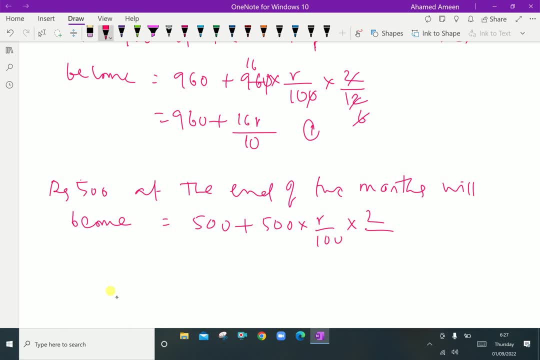 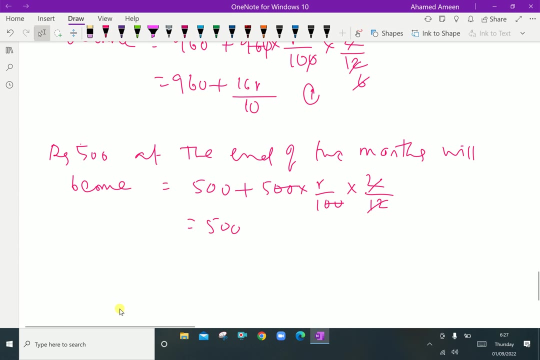 hundred into two months. 2 by 12. that means 2 by 12 is years. now by simplifying it become 500, 500 plus 5 off by this world for one month, not two months here, just first month. so it is boy, all by 12. very beautiful. 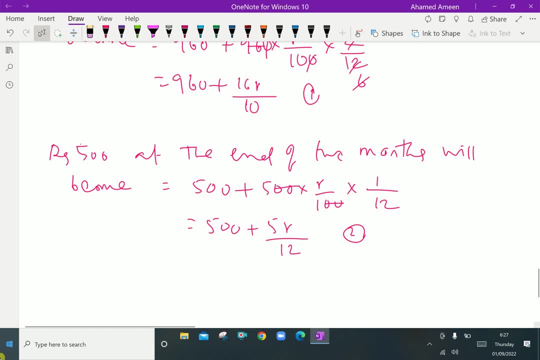 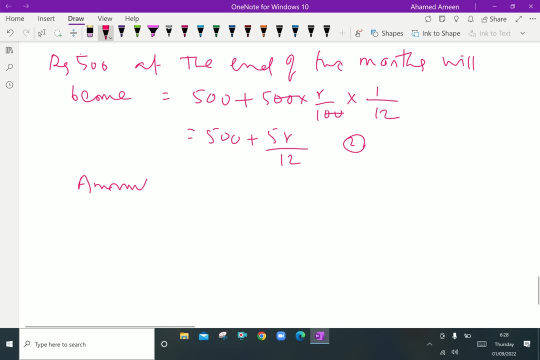 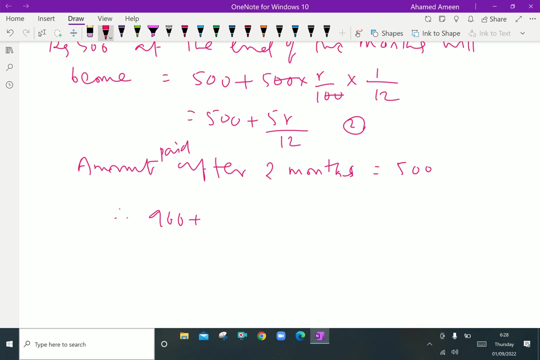 amount after two months. come on, two months. ok, that is half amount. muy bien, ok, that is half amount. come on, okay, thank you, okay, thank you, okay, thank you. amount paid after 2 months is 500, therefore, which? therefore, you can see the equation: 960. this, that is from. 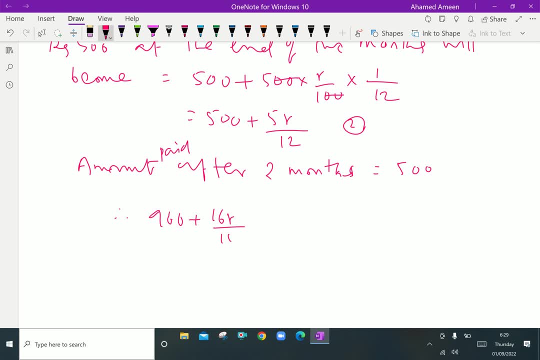 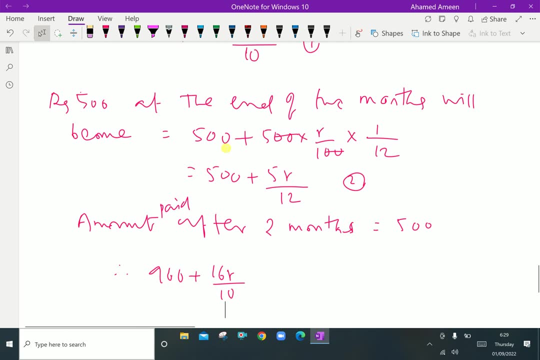 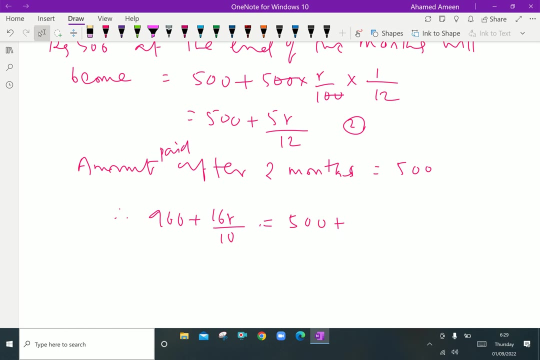 equation: 116 R by n, that is your 960 plus 60 R by 10, which is equal to 500 plus 500 plus 5R plus 12, 500 is the second month. then amount paid after two months is 500, so the 500 is added. 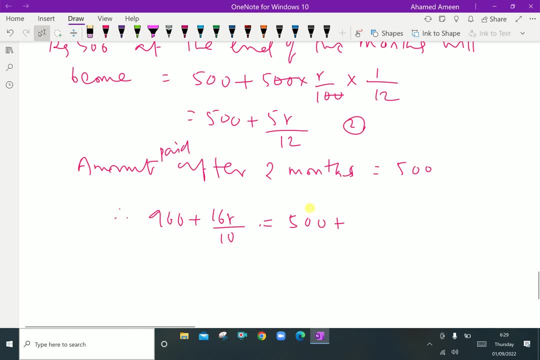 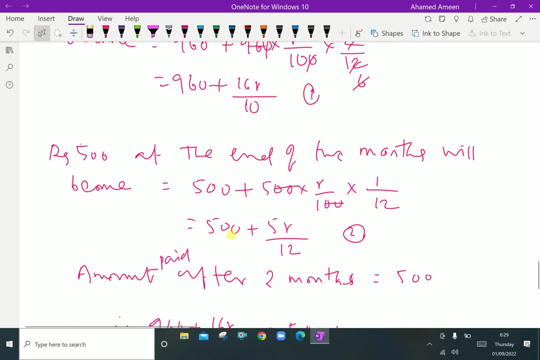 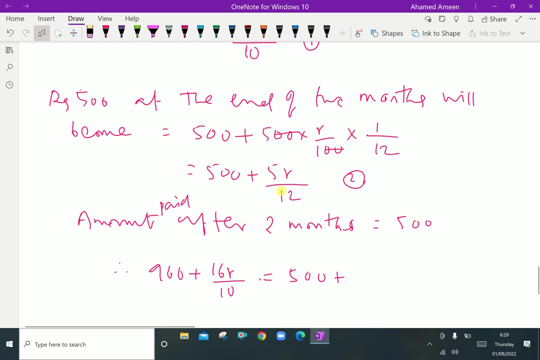 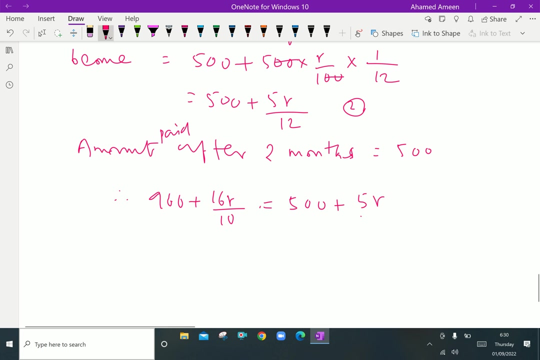 here. that is 50 R by 10. that is 500 plus the 5R plus 12, 5R over 12. so we are there. here. that is 500 plus the 5R plus 12, 5R over 12. so we are there. 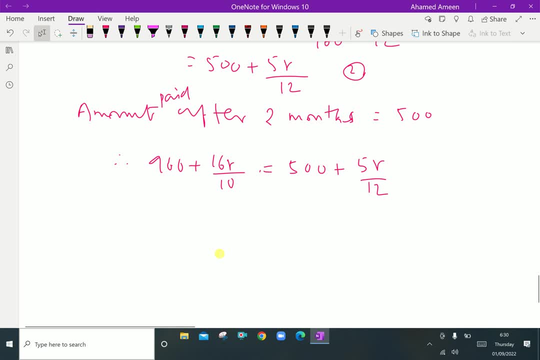 like what? 500 then, which is equal 16 R by 10 minus 5R by 12, equal 500 plus 500 minus 960. look at here: this 16 R minus of the set is 5R by 12, equal 500 plus 500. 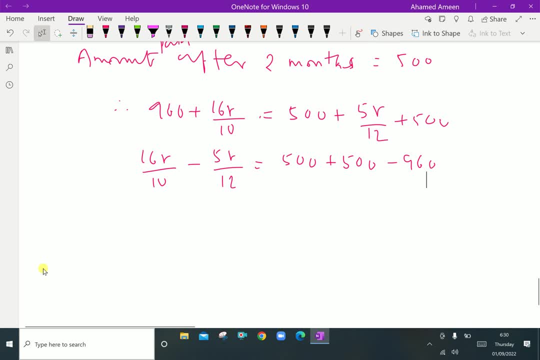 minus 960, which is equal. by taking LCM here. 60 is an LCM for 10 and 12, that is 16 to 16 is 96R. minus 5 into 5 is 25R, is equal 500 plus 500 is 1000. minus 960 is 40.. So 96R. 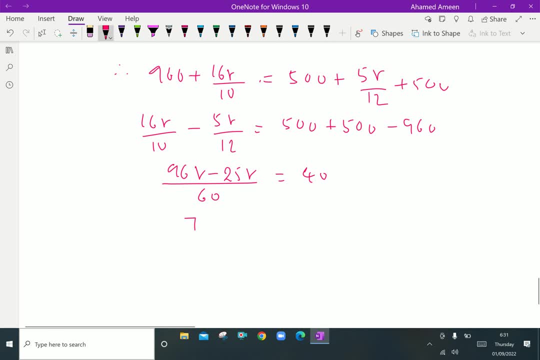 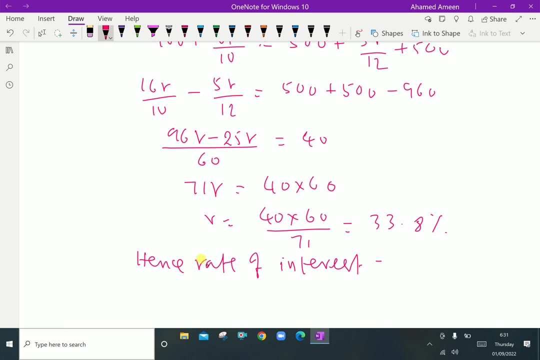 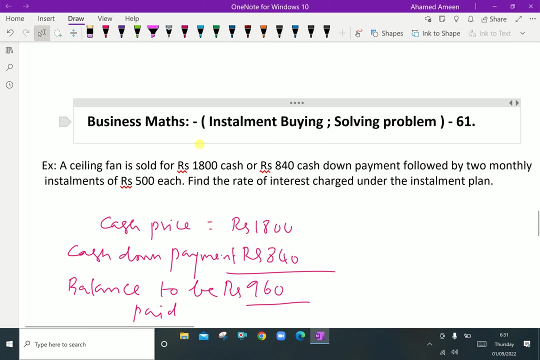 minus 25R is 71R equal 40 into 60,, then R equal 40 into 60 over 71,, which is approximately equal 33.8%. Therefore, hence rate of interest, and rate of interest equals 33.8%. So for I had done here in Business Mathematics. 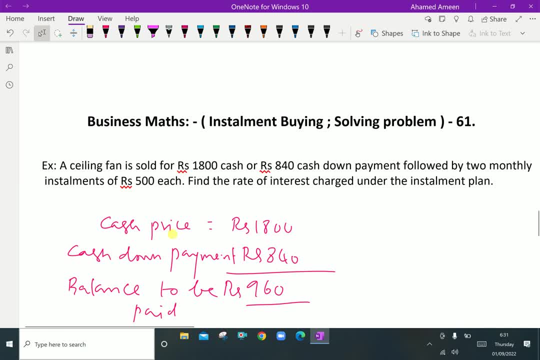 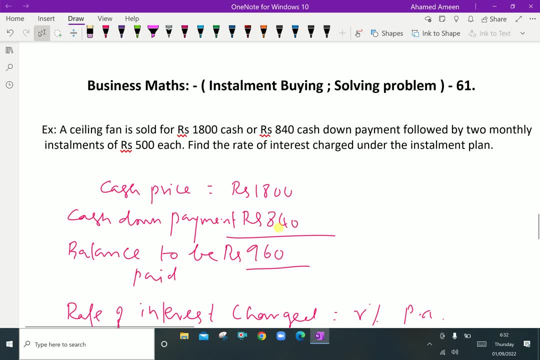 installment paying- solving problem here- the cost of ceiling payment if immediate payment, full payment, is 1800, but case down payment is 840.. So the balance to be paid is 969.5.. So this is the balance. 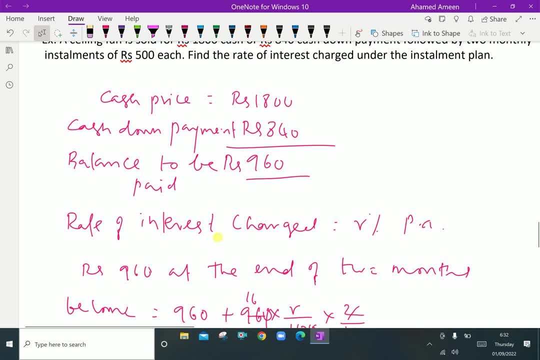 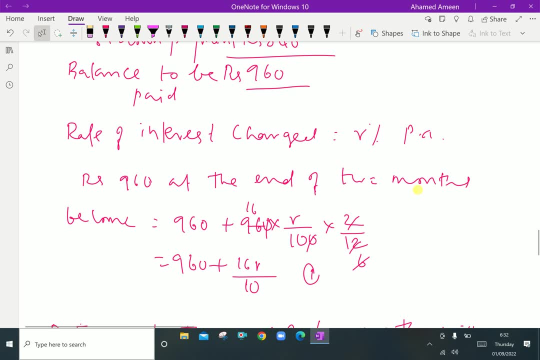 So this is my investment. This is the return rate of interest charge. it is r percent per annum. we have to like it here. rupees 960 at the end of two months become 960 plus 960 of r percent. that is 960 into r percent for two months. that is. 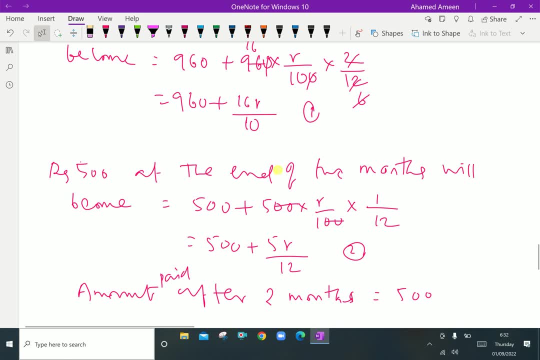 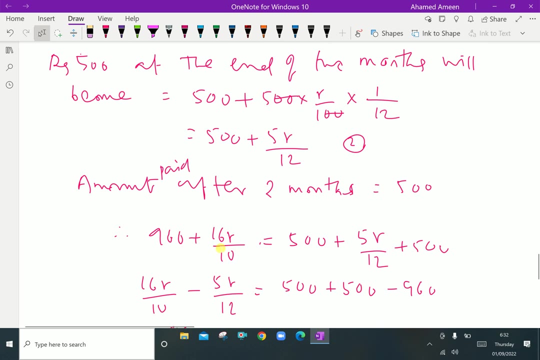 simplifying here. then rupees 500 at the end of two months will become 500 plus 500 into r by 100, 1 over 12. so it becomes like simplification that the amount paid after two months is another 500, so that equating both, that is, 960 plus 16, r by 100, is equal 500 plus 5, r by 12 plus 500 from. 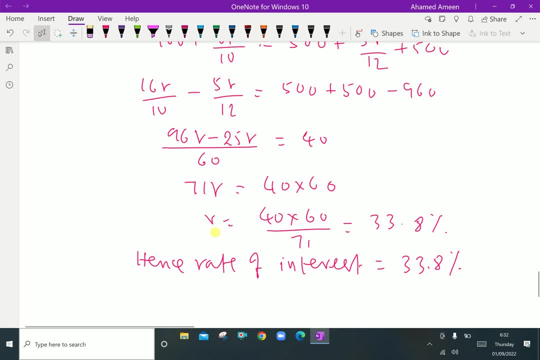 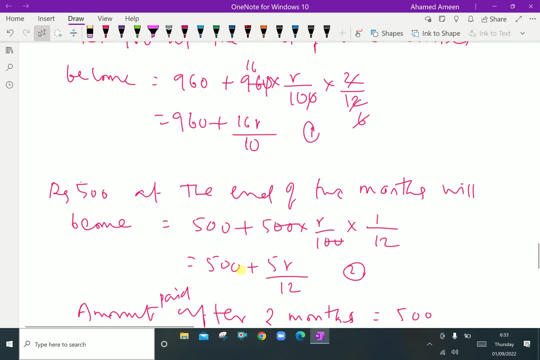 this we calculate. r percent is 33.8 percent. we have done. please subscribe our youtube channel you.